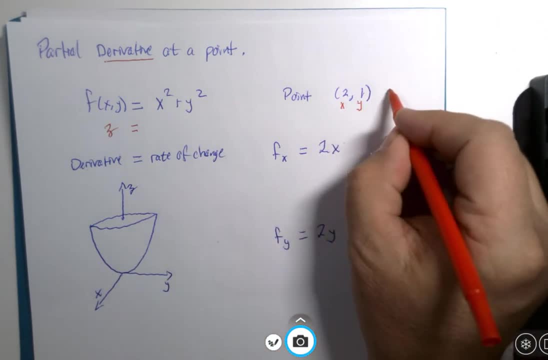 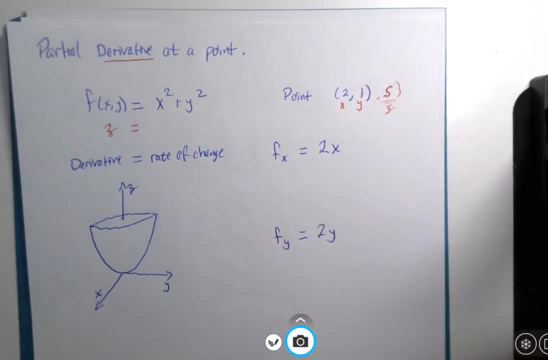 could certainly find the Z value to go with it. it would be 5. if we were really curious what the Z value was. it's 5, that's a 5. so I would go two units in the X direction and I would go one unit in the Y direction and 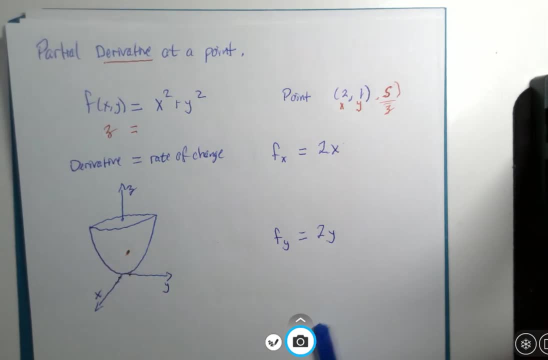 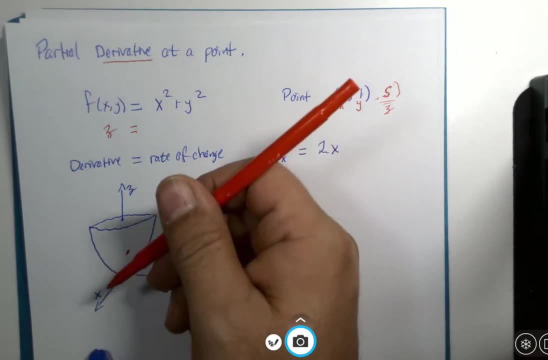 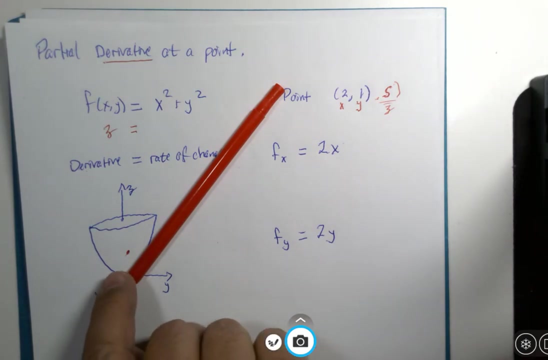 it would be this point right here. well, what this means is: what is the rate of change if you were pointed in the X direction? how steep would that graph be if we were kind of climbing up the side of it? and then the partial derivative with respect to Y is the same thing. what? 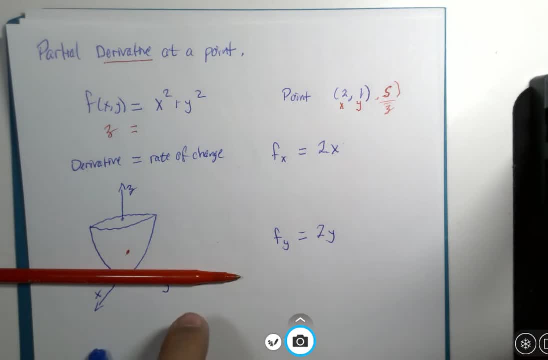 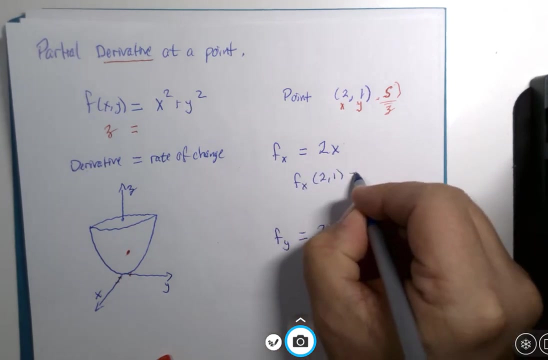 would it be like if we were aiming in the Y direction? what's the change of aiming in that direction? and and so let's give a number to this. the partial derivative with respect to X at the point 2, comma 1. well, if X is 2 2 times 2 is 4. 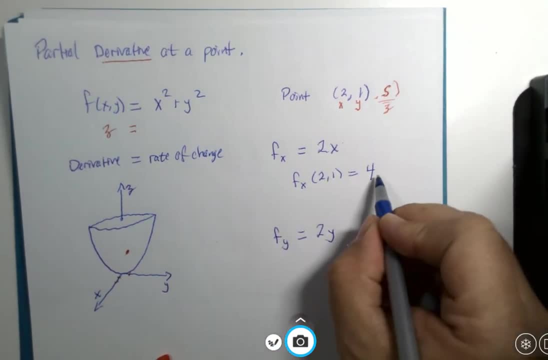 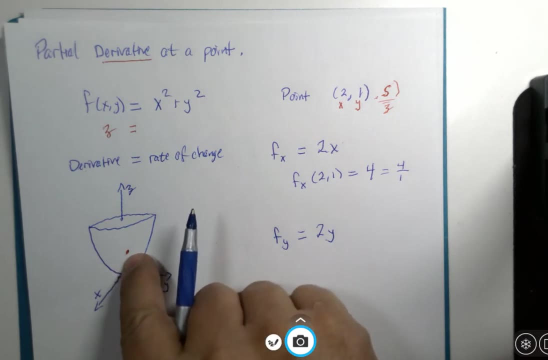 well, if X is 2, 2 times 2 is 4, and we could think of 4 as 4 over 1. what that means is, if you were to go in the X direction, the steepness here would be up 4 in the Z direction and over 1 in. 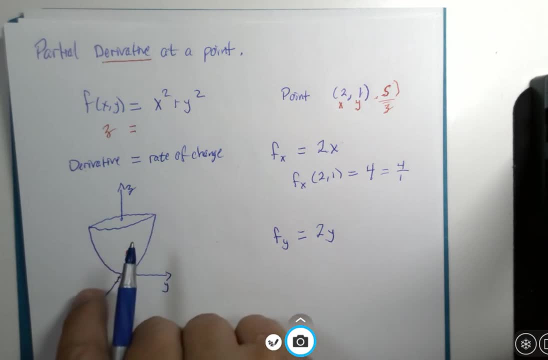 the X direction, the partial with respect to Y. I should put parentheses here. 2 comma 1. my apologies, let's see a 2 times 1 is 2 or 2 over 1. at this place in the curve it's not as steep. in the Y direction the change isn't as great now. 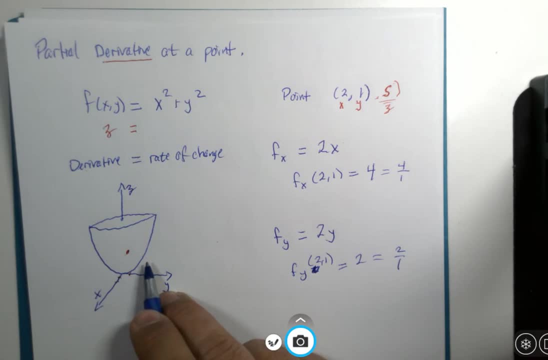 the book has much better diagrams than I'm providing you here, and if you just like to calculate and you don't really mind understanding what's going on, but fine, go ahead and use it. can calculate these. they're not really difficult at all to calculate, but you just need to know that. 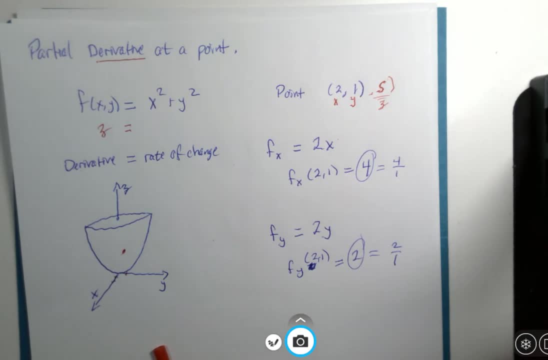 in the real world, after you leave a course, somebody uses this, this derivative, to measure a rate. so right now we're looking at it as a partial derivative. we're looking at the rate if we go in one direction in particular, either x or y. so let's see one more sample that we cannot graph at all. 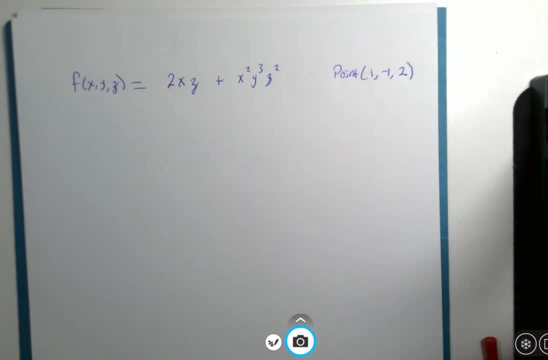 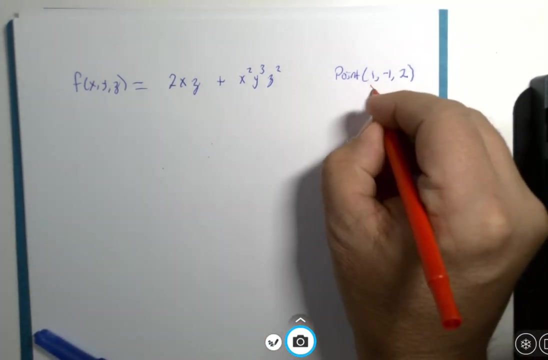 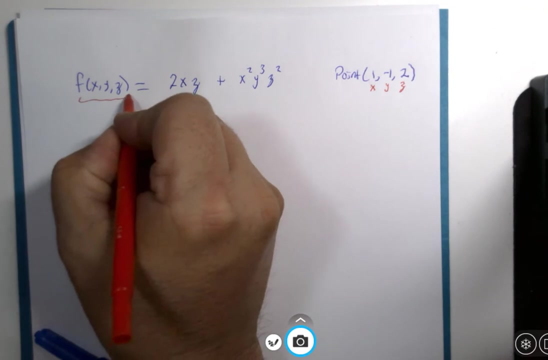 f of x, y and z is 2 x, z plus x squared, y cubed, z squared, and our given point x, y and z coordinates are 1 and negative, 1 and 2, and that means the output is a completely different variable. our book happens to use the letter. 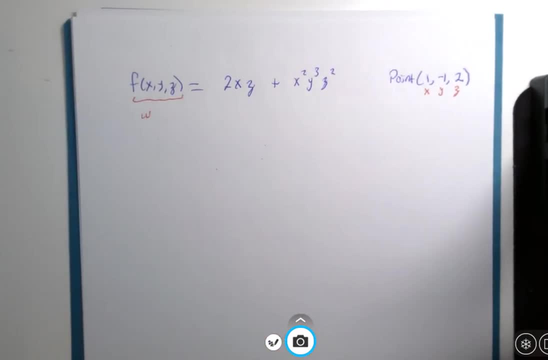 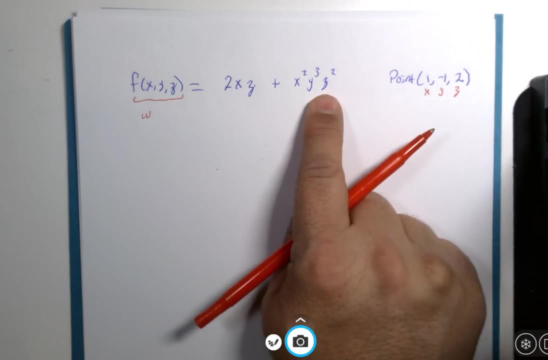 um, w, sometimes for a fourth dimension. but remember, in the real world they wouldn't probably use any of these letters unless it made sense for the real world problem. so we're going to do the calculation for one of these derivatives first and then i'm going to see if i can't give you a possible. 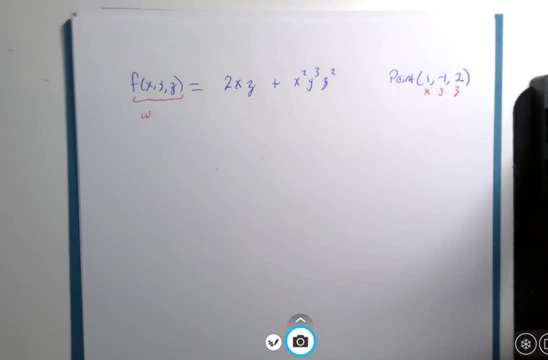 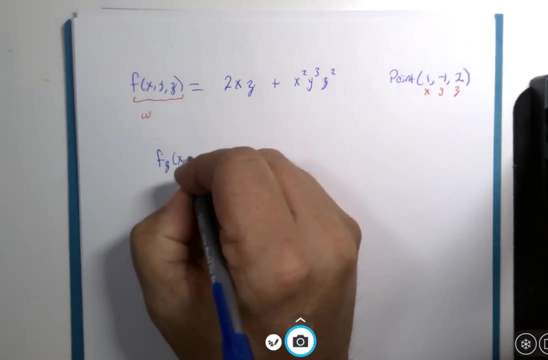 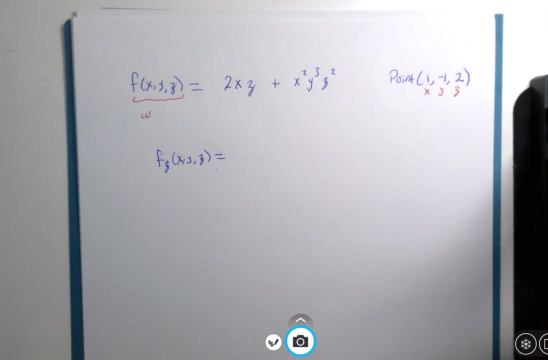 interpretation of that number. let's just do one calculation with this, the partial with respect to z, since i think i have done maybe one of these and combined in my previous segments, at least to this point in time, if z is the variable, the derivative z is 1, leaving you just. 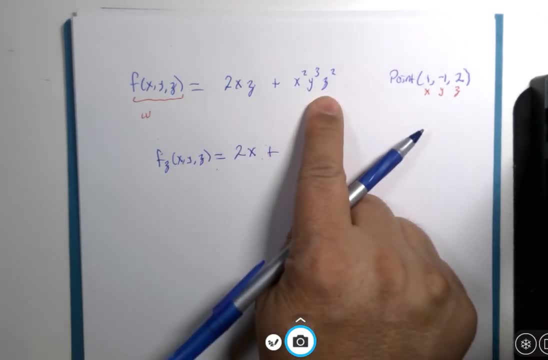 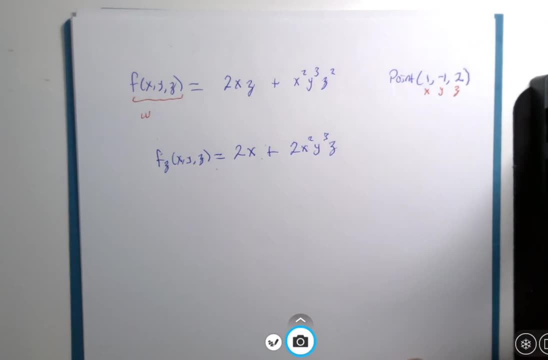 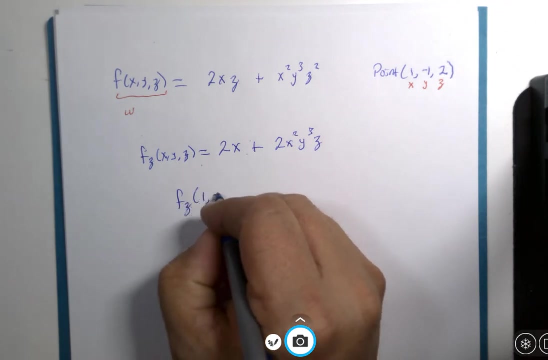 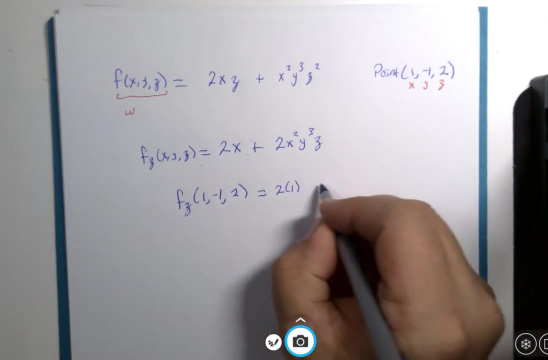 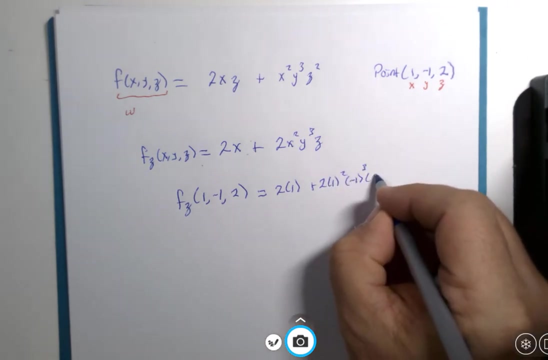 the constant 2x. if z is the variable here, you get 2 multiplied by x squared y, cubed z to the first. if we then do this and evaluate it at the point 1 and negative 1 and 2, let's see that's 2 times 1 plus 2 times 1, squared times negative 1, cubed times another 2. 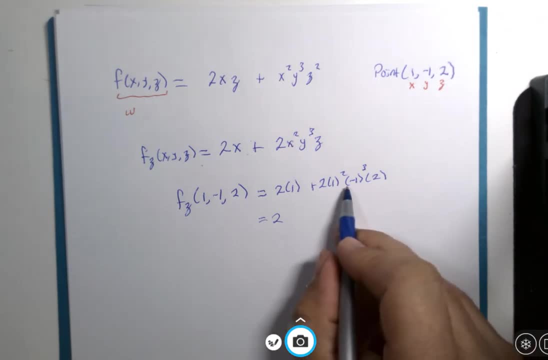 let's see here: it's 2, it's 4 negative, 4 negative, 2. i get negative 2.. so what kind of a rate of change is this? what does it look like in the fourth dimension? i don't need you to have the 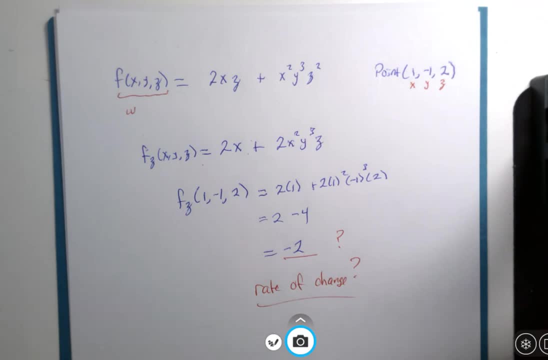 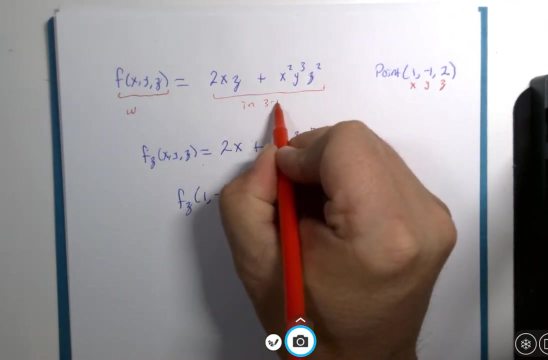 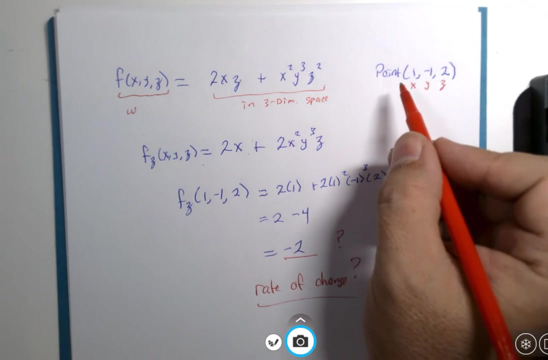 ability to try to imagine in four dimensions. uh, my own skills there are severely lacking. i can give you a possible meaning for this. so what if this was a measurement in three dimensional space? we have x, y and z. we have a location in space. and what if the fourth variable measured? 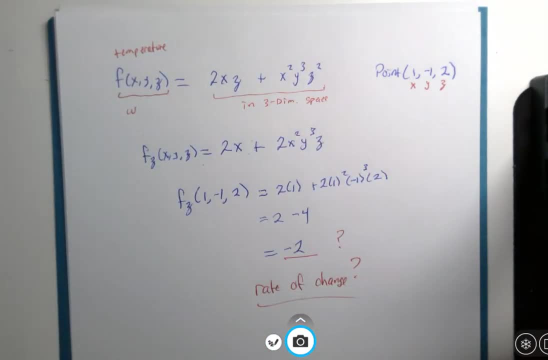 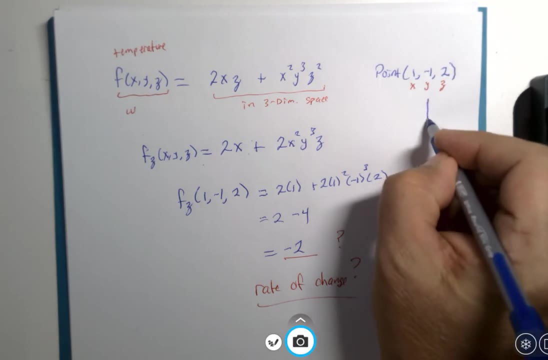 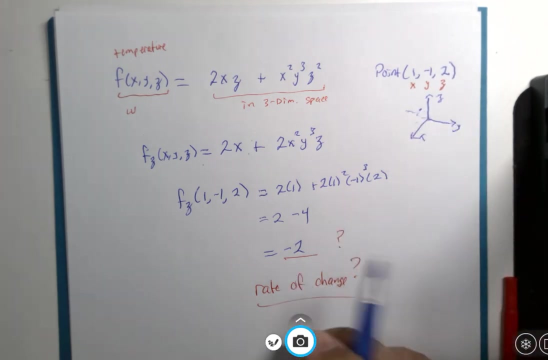 temperature at a place in space. What this means is if you were to go to the point where X is 1, Y, X, Z, X is 1, Y is negative 1, Z is 2, and then you would aim in the Z direction. your temperature is going. 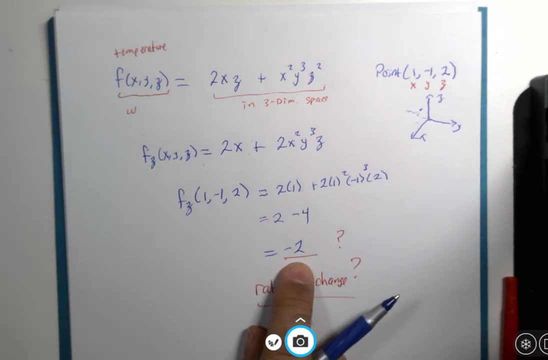 to drop by 2 degrees per unit of Z, Your temperature would be going down. If this was a positive number, your temperature would be going up, And then, if you did the X partial derivative, you'd see what would happen to the temperature. 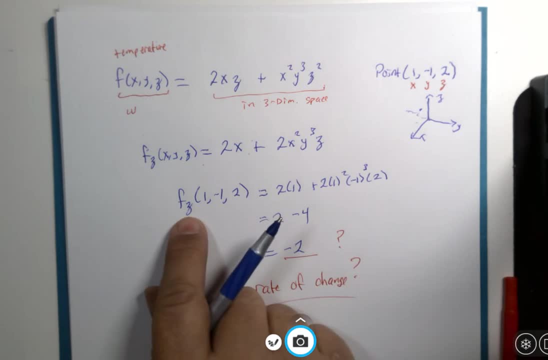 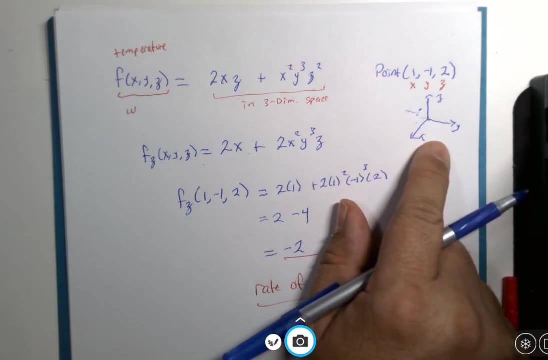 if we went in the X direction And the Y partial derivative? what would happen to the temperature if we went in the Y direction? And then later this chapter, we'll say: well, what if I want to go in a different direction? 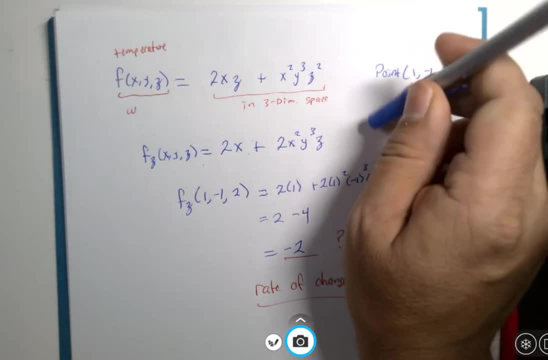 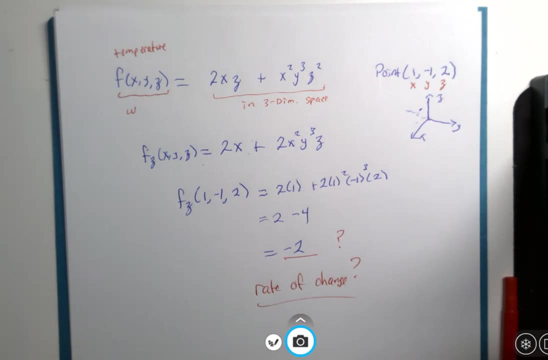 What if I want to go that way, Or if I want to go this way, Or if I want to go that way, But we are not quite ready for that yet. We need a few more tools and a bit more experience. All right, 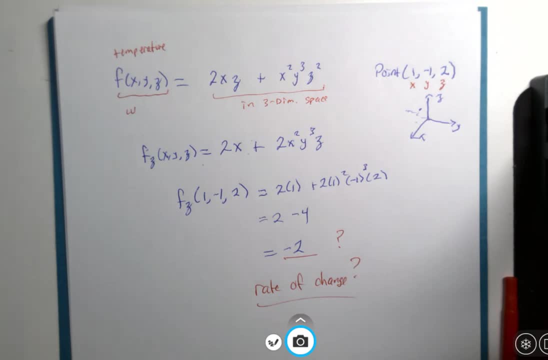 We've got a little bit more to do with the basics of partial derivatives, so stay tuned.